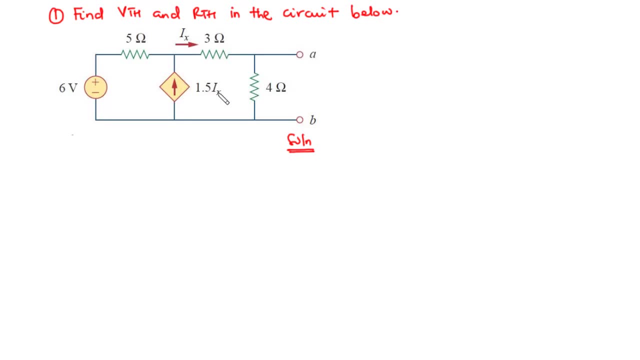 Now to solve a circuit using Thevenin's theorem. we know the first thing is to deactivate the independent sources. Now we are going to deploy that here. So you know that whenever you deactivate a voltage source, then you represent that with a short circuit. And then, whenever you deactivate a current source, 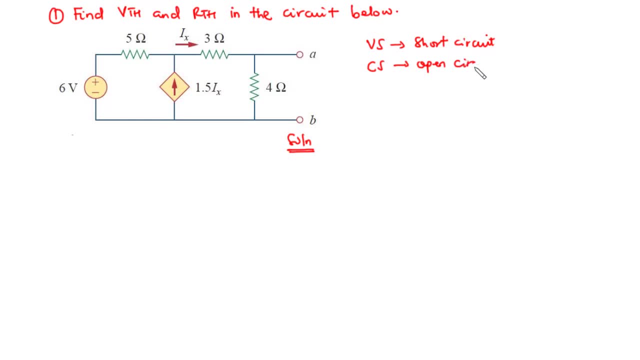 you are going to represent that with an open circuit. So that is the first thing we are going to do: We are going to redraw this circuit, deactivating the 6V source. So, after redrawing the circuit deactivating the 6V source, we are going to move on to find Rth. 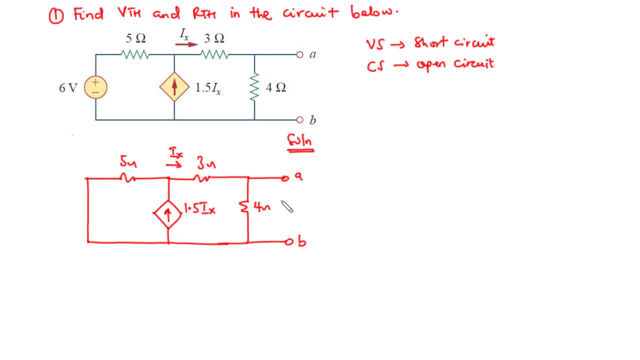 Now to find Rth, the first thing is to introduce either a voltage source or a current source in between the two terminals. Now you can either introduce a voltage source or a current source. Now, for the sake of simplicity, we either introduce a 1V source or 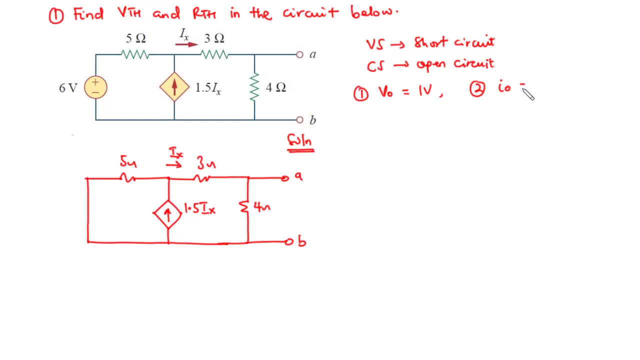 a 1V source. So we are going to introduce a 1A current source. So, either a 1V source or a 1A current source. Now, the moment you introduce V0, which is 1V, then you want to find the value of I0. 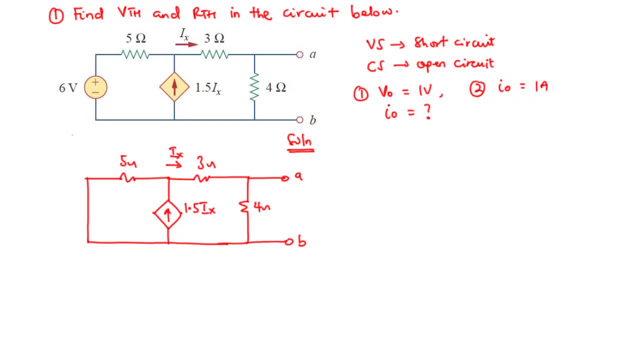 And then whenever you introduce I0, which is 1A, then you want to find V0.. Now, at the end, using the 1A current source, you can find the Rth, which is the TNR. So we know that V is equal to IR. So if you want to find, 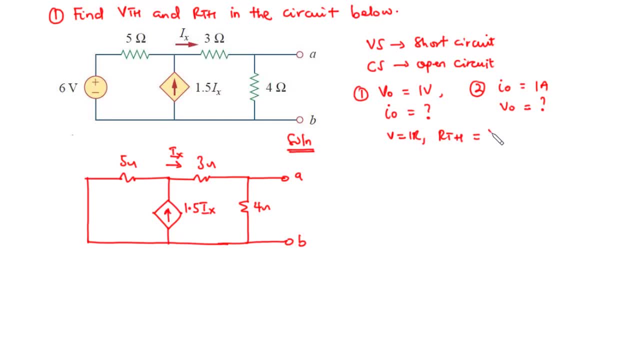 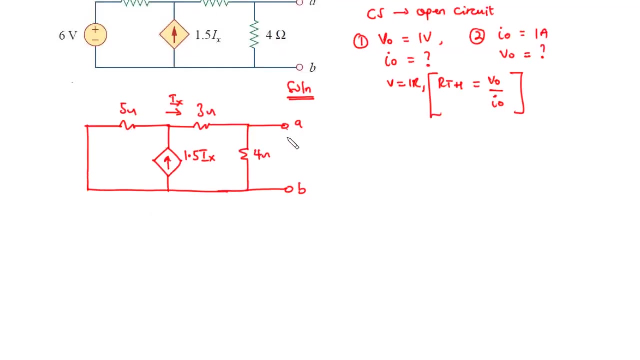 the TNR. it is nothing but V0 over I0.. This is how to find the TNR, So we are going to use or deploy that approach here. In this lesson we are going to introduce a 1V source, So you can also solve this example where you introduce a 1A current source At the end. 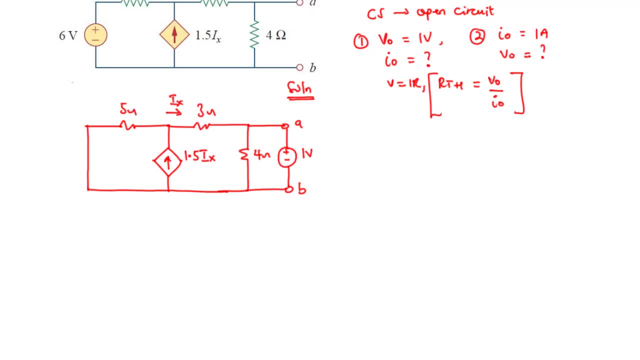 you are going to obtain the same values. So after introducing a 1V source, let's try to do current distribution in this circuit. So you have this dependent source having current 1.5IX moving toward this node, And then you have been told that you have IX leaving. 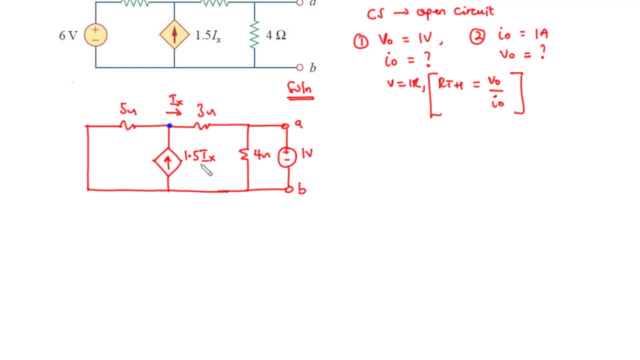 leaving in this direction. therefore, you have 1.5 minus 1 also leaving in this direction. so 1.5 minus 1 is 0.5. so we have 0.5 i x also leaving in that direction. and then let's assume that 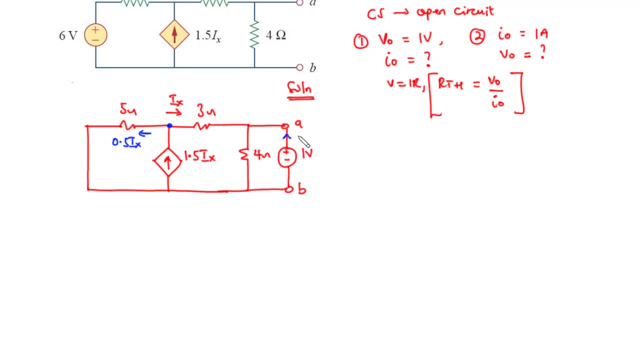 we have the current produced by this voltage source to be i naught. now we have i x flowing in this direction and then i not also flowing in that direction, so they meet at this node, and then the sum of the two currents, that is i naught plus i x flows in this branch, so the current 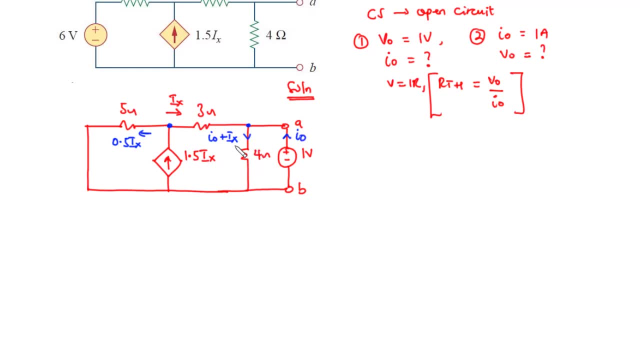 in the four ohms resistor is, i naught, plus i x. now let's try to find the value of i x. and then i naught so from kvl. we know that the sum of the source virtue does kill the current, and you will be able to see it now and then this value. 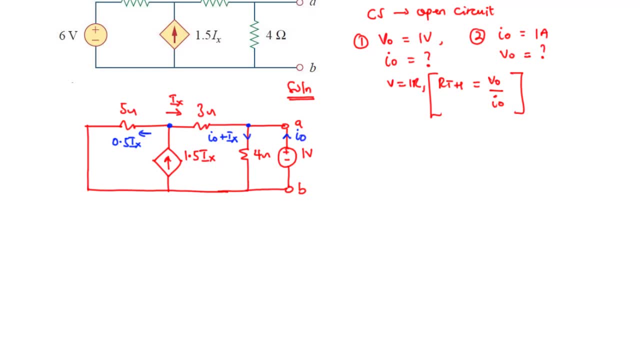 is equal to the voltages dropped across the loop. so let's consider loop one. so we are going to choose this to be loop one. so we have the source voltage to be one volts and that is equal to. we are taking the anti-clockwise direction. so 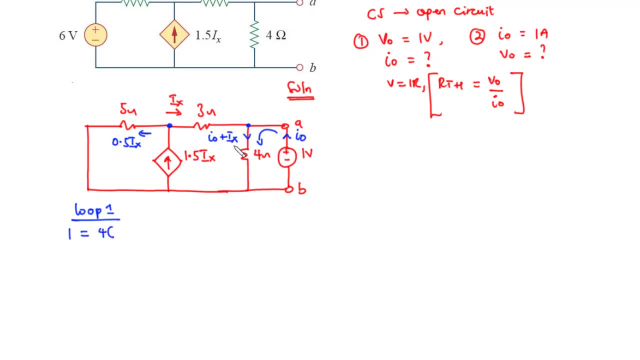 we have this to be equal to four times the value of current in this branch is: I naught plus IX. I naught plus IX. now let's call this equation one again, let's move on to another loop. we call that loop two. so in loop two we are going to. 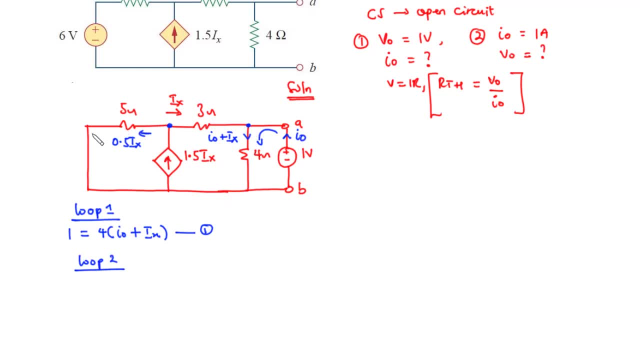 consider this whole bigger loop. we are going to consider this whole bigger loop and then, moving in the clockwise direction, here we have the source voltage to be zero. okay, we don't have any voltage source. okay, we don't have any voltage source. okay, we don't have any voltage source. 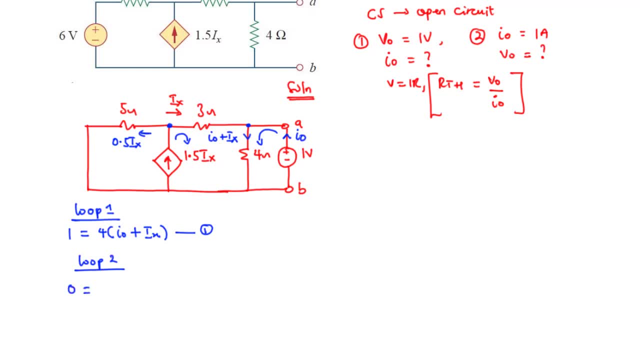 so the source voltage is zero, so we have zero equals. now we are taking the clockwise direction, so we have IX flowing through three ohms, so we have three times IX, plus moving in the clockwise direction, we have, I naught, plus IX flowing through four ohms. so plus four into brackets, I naught plus IX. 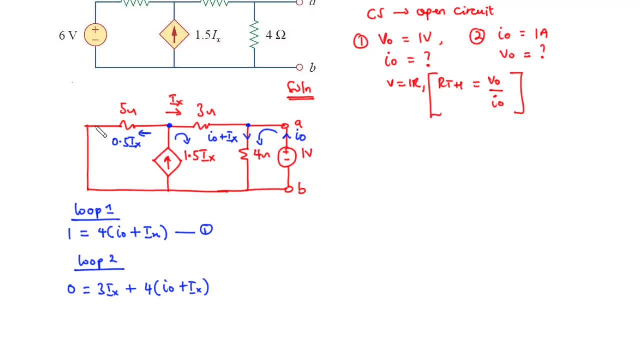 and then, still moving in the clockwise direction, you have this direction and then, still moving in the clockwise direction, you have this direction opposing 0.5 IX. so it becomes negative 5 value of resistor times 0.5 IX. now let's try to simplify this. so we have 0 equals 3 IX plus now from equation 1, you 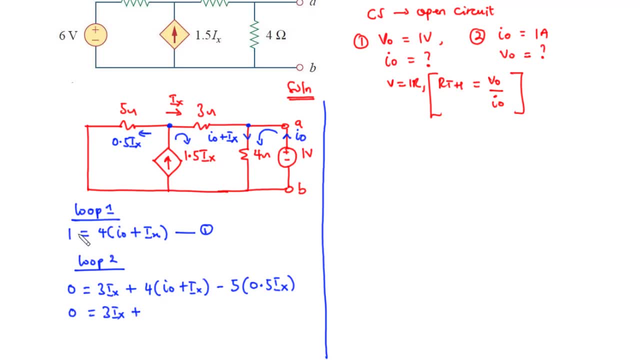 have 4 into brackets. I naught plus IX to be equal to 1, and that is exactly what you have here. so in place of this we are going to have 1 and then minus 5 times 0.5 is 2.5, so 2.5 or negative 2.5, IX. now we can combine these two: 3 and then. 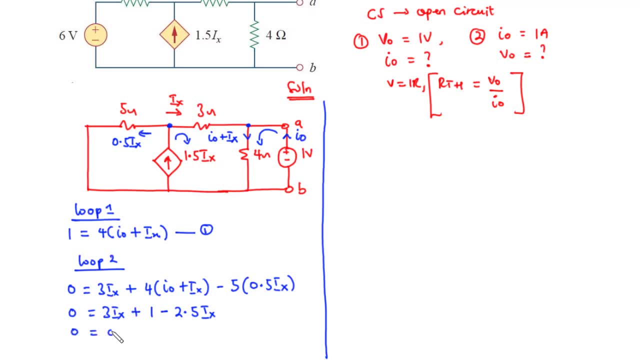 negative 2.5, so that becomes 0.5 IX plus 1. now we transpose 1 to the left hand side, so that we have 2.5 to the left hand side, so that we have 2.5 to the right hand side, so that we have 2.5 to the left hand side, so that we have: 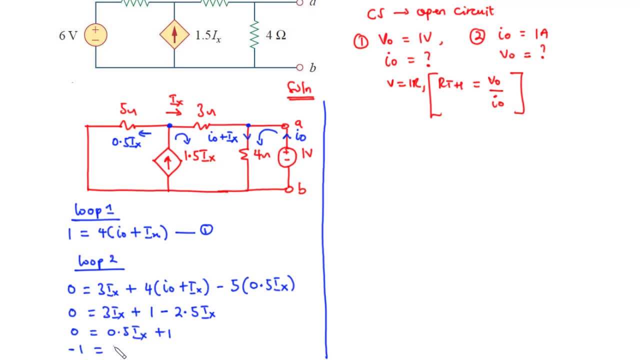 1 equals or negative 1 equals 0.5 ix. okay, so we have 0.5. ix equals negative 1. we divide through by 0.5- 0.5, and then we have ix to be equal to negative 2 amps. so this is the value of ix. now. 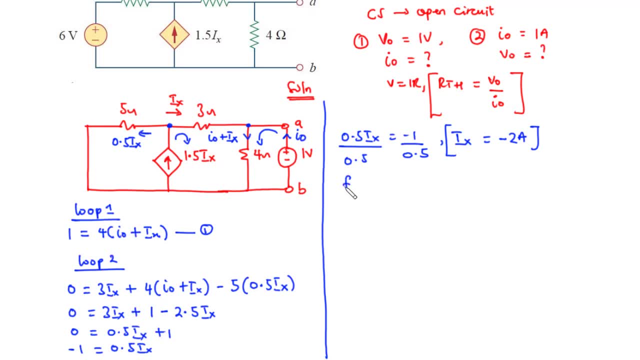 the focus is to find the value of i naught. so from equation 1. from equation 1 we have 1 equals 4 into bracket i naught plus ix, which is negative 2. so this becomes 1 equals 4. i naught, and then 4 times negative. 2 is negative 8. so we transpose negative 8 to the left hand side. 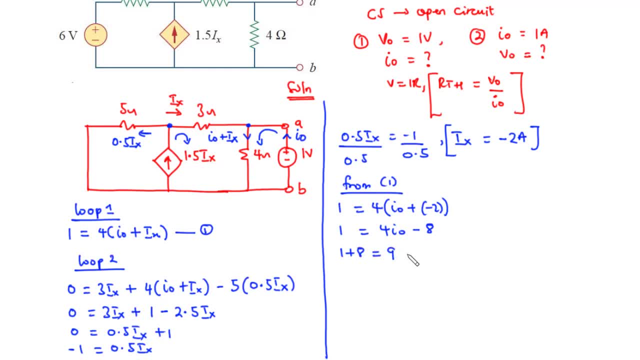 we have 1 plus 8, which is equal to 9, and that is equal to 4. i naught we divide through by 4, by 4, and then we have i naught to be equal to. now, 9 over 4 is 2.25. so this is the value of i naught. 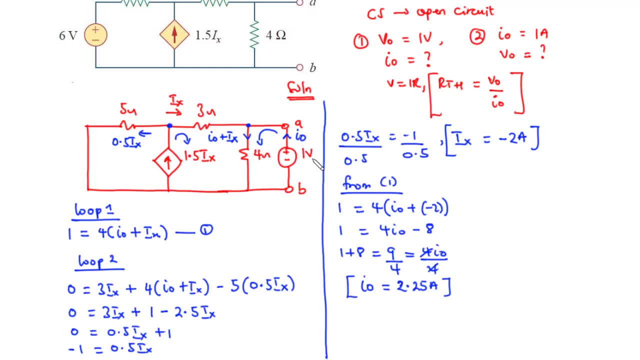 now, since we have the value of v naught, which is 1 volt, and then i naught, which is 2.25 amperes, then what this probability means is that we can find rth, that is, the resistance in between the two terminals, or? 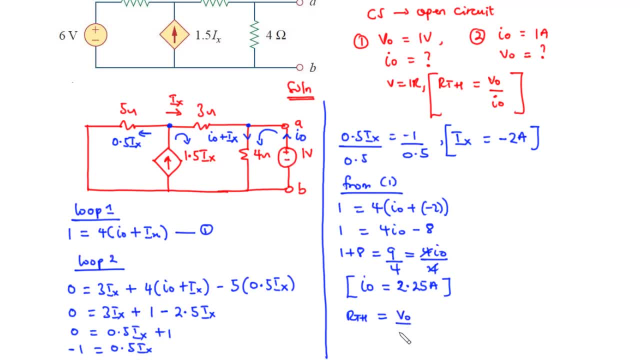 the terminus resistance to be equal to v naught over i naught, and that is equal to 1 over 2.25. now, 1 over 2.25 is equal to 0.4444 ohms. therefore, we have rth to be equal to 0.44 ohms, that is, to two decimal places. so now, after finding or getting the value, 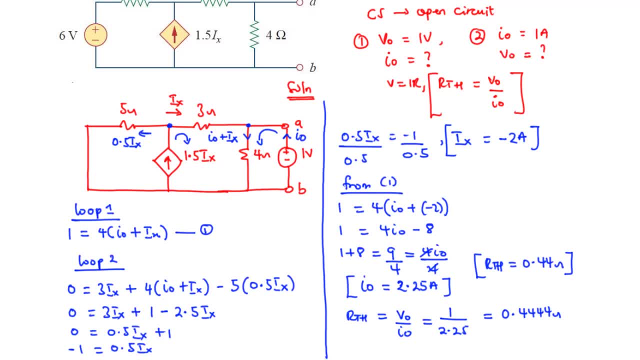 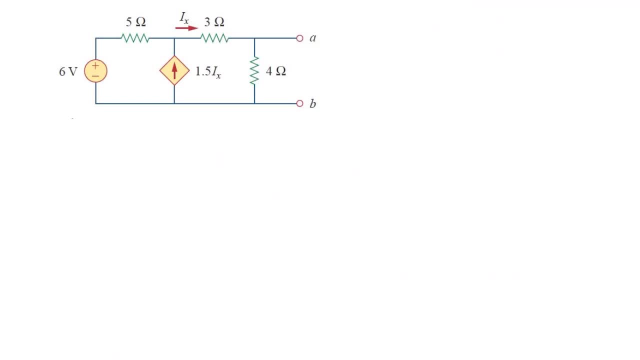 of rth. let's move on to find vth. so to find vth- that is the terminus voltage- we need to revisit the original diagram. now what we are going to do is we have our vth here, which is the open circuit voltage. then the next thing we are going to do is to make sure we do current distribution. 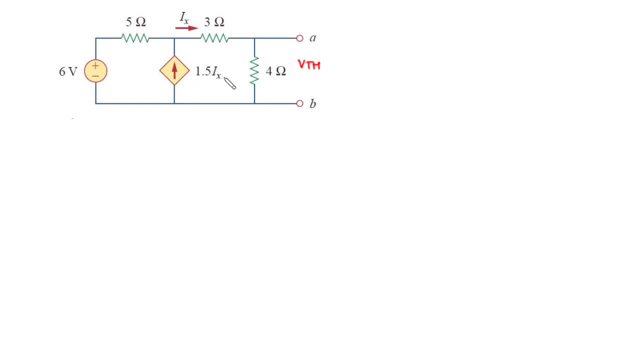 in the circuit. so we have 1.5 ix flowing towards this node. we have ix moving this way. therefore, we have 0.5 ix moving that way. notice that the moment you want to find the value of vth, you need to revisit the original circuit given in the question. make sure you don't eliminate any. 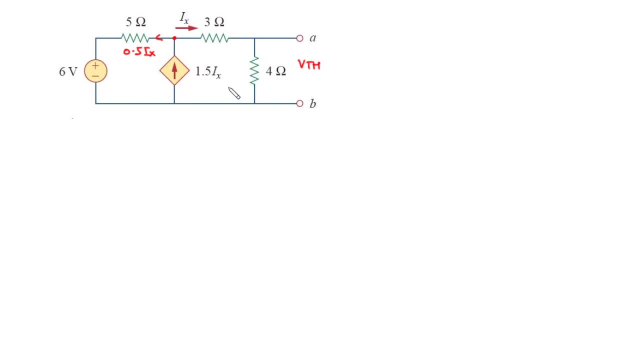 other circuit element in the original circuit. now let's try to consider this loop. let's consider this loop. so we are taking the clockwise direction. so, according to kvl, we know that the source voltage is equal to the sum of the voltages dropped across the loop. we have the 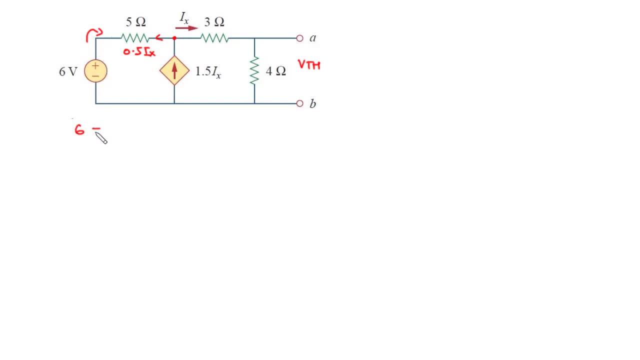 source voltage in this loop to be 6 volts. so we have 6 and that is equal to. now we are taking the clockwise direction. this is opposing the direction we are taking. therefore it becomes 0.5. so we have negative 5 times 0.5, ix plus. this is in line with the direction, so plus 3 times ix. 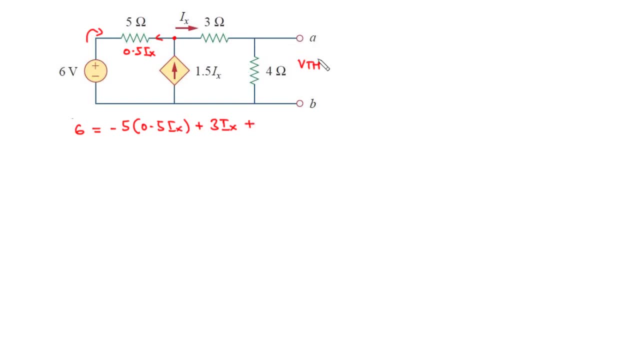 plus now, because we have an open circuit here, no current will like to flow in this direction. so all the current that flows through the three ohms will like to flow in this direction. therefore we have the same current, ix, flowing through this branch. therefore we have 4 ix and then we can find the value of ix. so let's simplify this. so we have 6 equals. 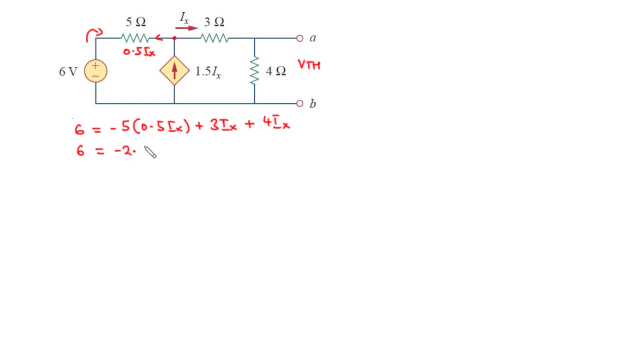 negative 5 times 0.5 is negative 2.5 times ix plus this becomes 7. ix now negative 2.5 plus 7 is 4.5. so we have 4.5. ix equals 6. we divide through by: 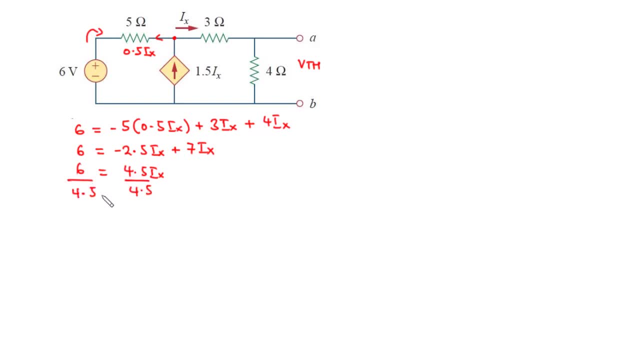 4.5 by 4.5, and then we have ix to be equal to 1.333 amperes. so that is the value of ix. now, remember that we have ix flowing in this branch, and then to find vth. vth is nothing but the. 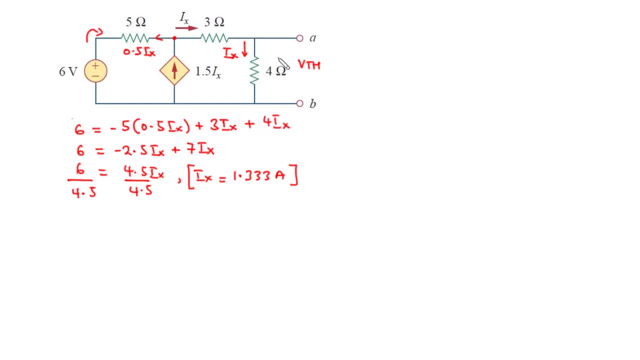 current flowing in this branch times the value of this resistor. so we are taking the anti-clockwise direction. we have vth to be equal to notice that this direction and that direction are in the same line. so we have vth equals 4 times ix and that is equal to 4 times. 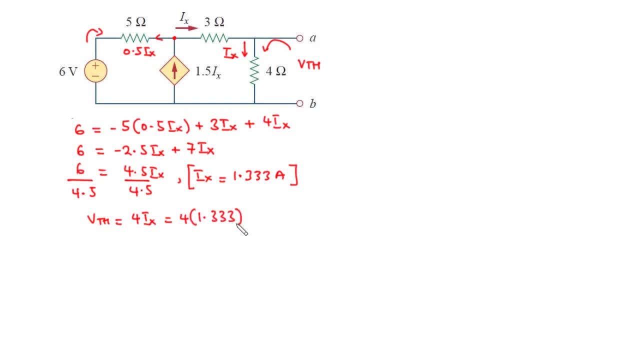 1.333 and then if you multiply the two values you have 5.332 volts. therefore we have vth to be equal to 5.33 volts to 2 decimal places. so we have vth to be 5.33 volts and then rth also to be 0.44 ohms. 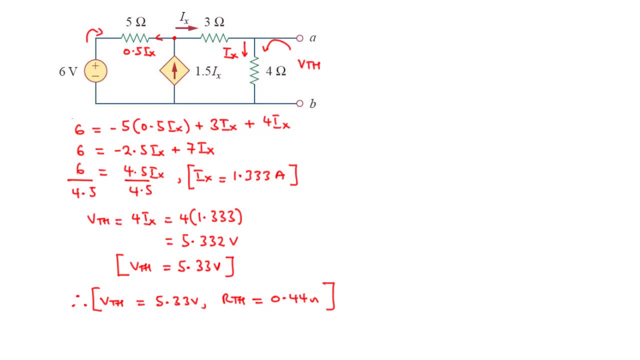 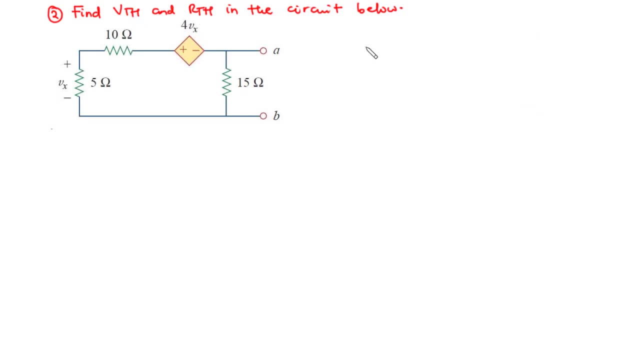 so now let's move on as we solve the second example. so in this second example we are also going to find and then RTH in the circuit below. Now in this problem, in this circuit we don't have an independent source. So straight away we are going to introduce either a 1 volt source or a. 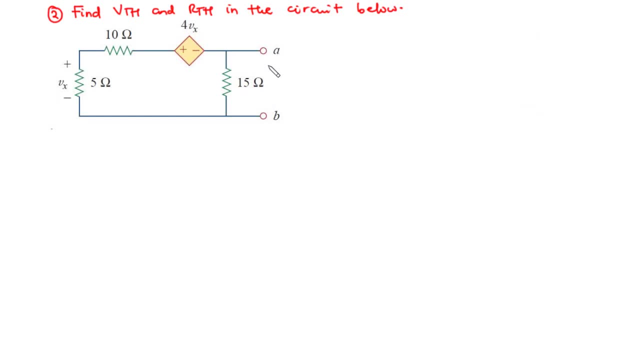 1 ampere current source between these two terminals. So let's introduce a 1 volt source between the two terminals, So we have a 1 volt source, and the current produced by this voltage source let's call that I0.. Now let's do current distribution, So we have I0 flowing towards. 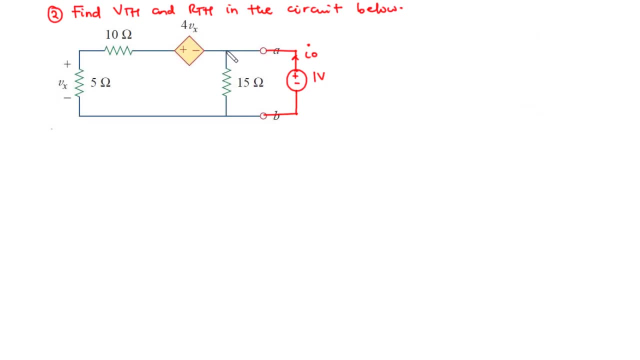 this node and then at this node we have the current splitting. Let's assume that we have current I1 flowing in this branch and the rest of the current, that is I0, between the two terminals. So we have a 1 volt source and the current produced by this voltage. 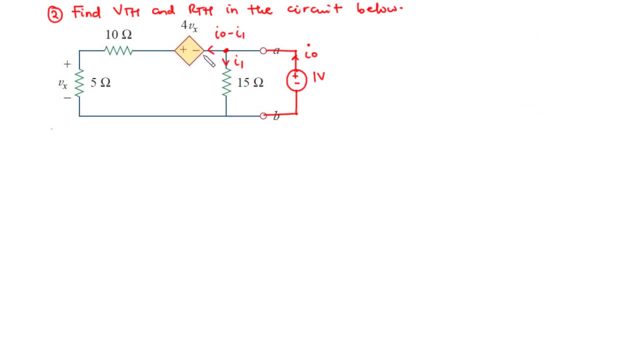 minus I1 flowing in in this direction. Now let's try to find the values of I0 and then I1.. So, considering this loop, considering this loop using KVL, we have the source voltage to be 1 volt and that is equal to the sum of the voltages. 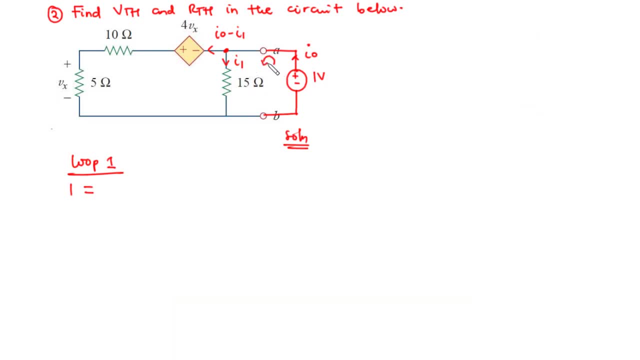 dropped across the loop. So, taking the anti-clockwise direction, we have 1V equal to I1, now we divide through by 15, by 15, and then we have the value of I1 to be 1 over 15 amperes. So this is the value of I1.. Now let's move on to find the value of I0. So this time we 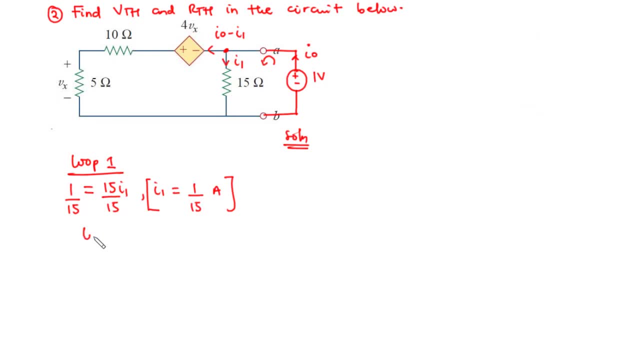 are going to consider this loop. Okay, so we call that loop 2, we call that loop 2, and then we are taking the anti-clockwise direction Again. use a PSV, Jurros. This is your local complex universities for childnet learning and but is called the C1 audience for this test. So let's try to do that. So when the water pushed into the wonderful, beautiful, beautiful base of the pathץ you area, niwellen, you were having a well-laden space behind thelast тысяч watt. It distracts a big amount of energy. This is. 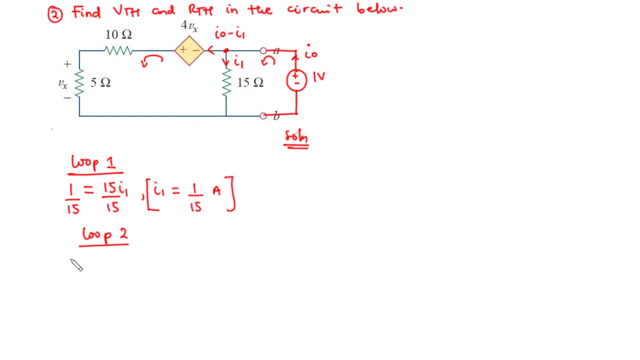 Again using KVL, we have the source voltage to be 4VX. That is equal to taking the anticlockwise direction. we have I0 minus I1 flowing through 10 ohms and then 5 ohms, So that becomes 10 plus 5.. 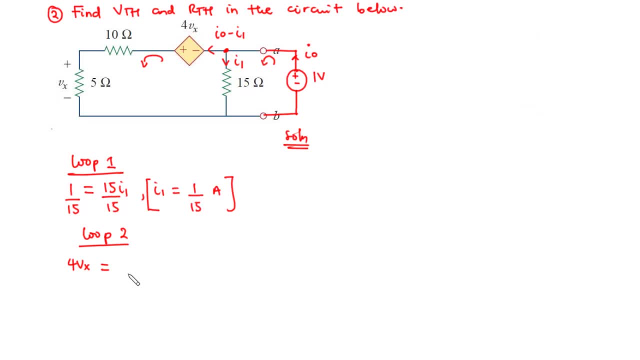 So we can just write 15.. Okay, so that is 15 times I0 minus I1.. And then here we have the current opposing the direction. So that's going to be negative 15 times I1.. Now we have VX. 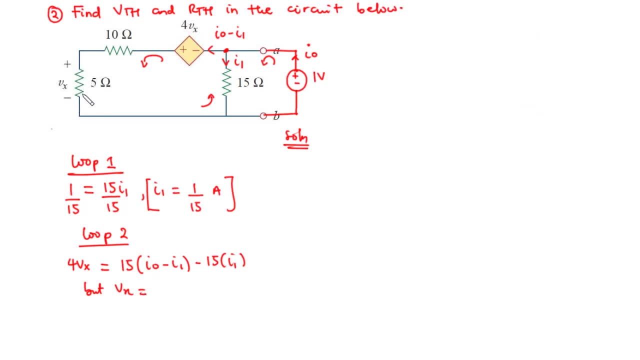 That is the voltage across this resistor And that is given by the value of current. We have the current flowing through this resistor times the value of the resistor. We have the current flowing through this resistor to be I0 minus I1.. Therefore, we have VX to be 5 times I0 minus I1. 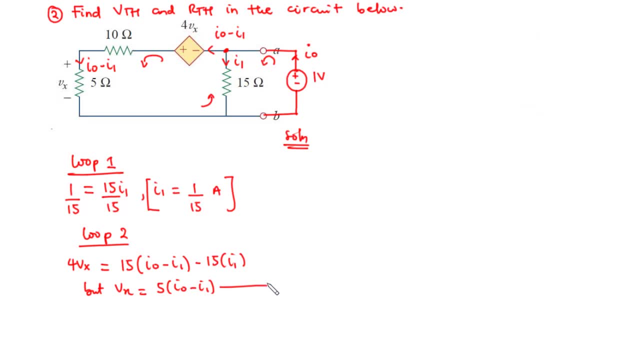 Okay, so we are going to substitute that into this equation So that becomes: we have 4 times in place of VX, we have 5.. That is equal to: let's try to, I mean, expand this. So we have 15 I0 minus 15 I1 minus 15 I1. 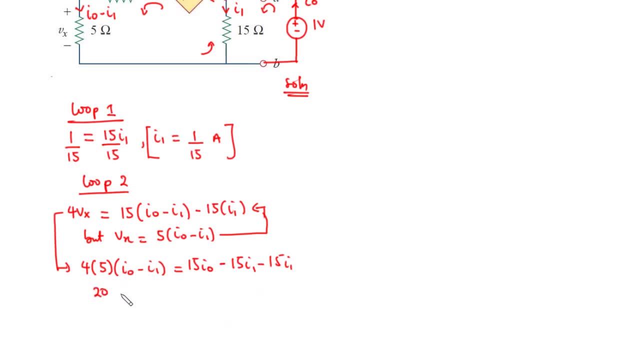 So on the left-hand side we have 20 I0 minus 20 I1, equals 15 I0 minus 15 I1.. Now we are going to transpose 15 I0 to the left-hand side and then negative 20 I1 to the right-hand side. 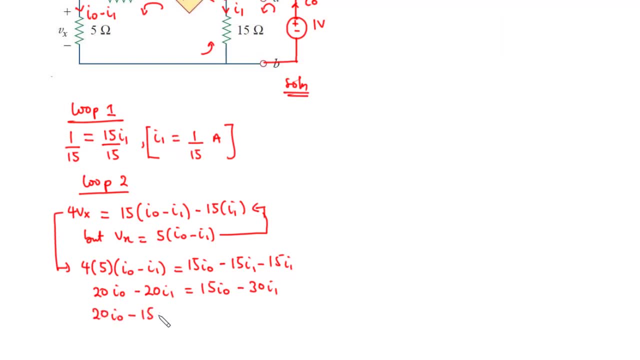 So we have 20 I0 minus 15 I0 equals negative 30 I1, and then plus 20 I1.. Now on the left-hand side we have 5 I0, and that is equal to on the right-hand side. 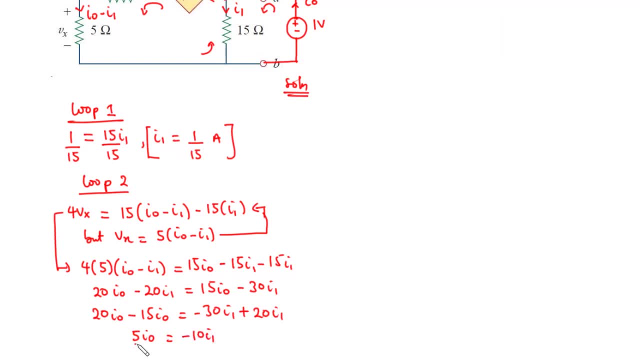 we have negative 10 I1. Now we can divide through by 5, so that we have: I0 equals negative 2 I1. So I0 is equal to negative 2. We have I1 to be 1 over 15.. 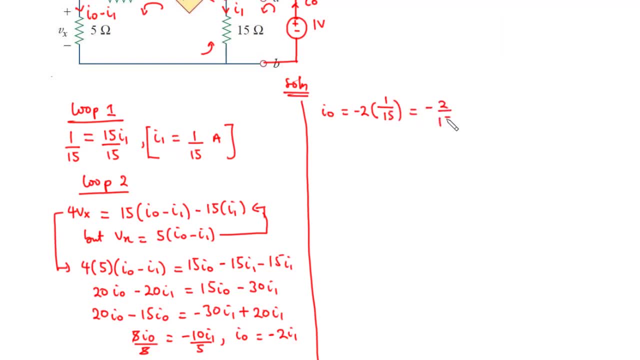 So that becomes negative 2 over 15.. So that's it. So that is the value of I0, negative 2 over 15 amperes. Now, since we have the values of V0 and then I0, we can find Rth. 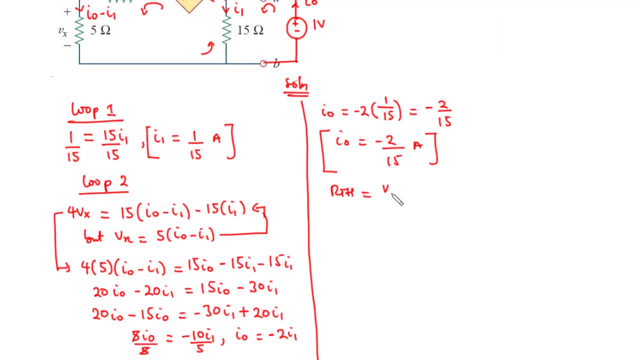 So we have Rth to be equal to V0 over I0.. We have V0 to be 1 divided by I0, negative 2 over 15, and that is equal to 1 times the reciprocal of this. So that's it. 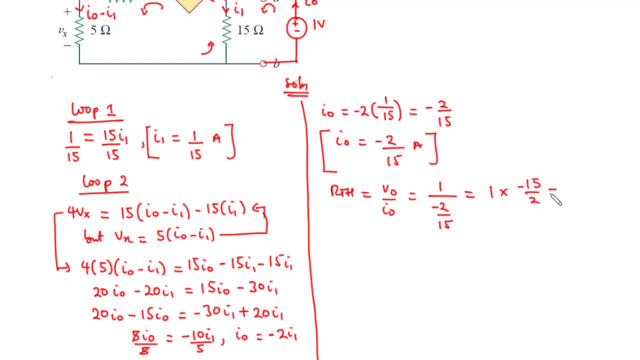 So negative 15 over 2, and that is equal to negative 15 over 2.. Negative 15 over 2.. Now, negative 15 over 2 is equal to negative 7.5.. Now, whenever you get Rth to be negative, what this primarily means is that the circuit is rather supplying power. 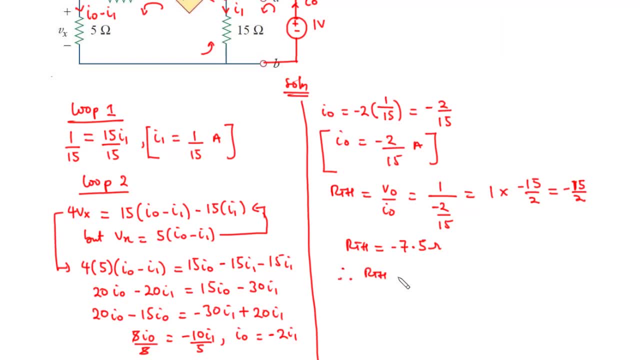 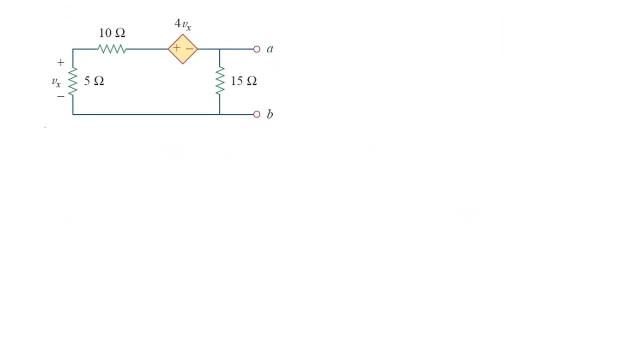 Therefore we have Rth to be 7.5 over 2.. That means the voltage is going to be higher than the voltage giving in the problem. Let's see the value of Rth to be 1 over 15.. So Rth to be 1 over 15 is equal to negative 4 over 1.. 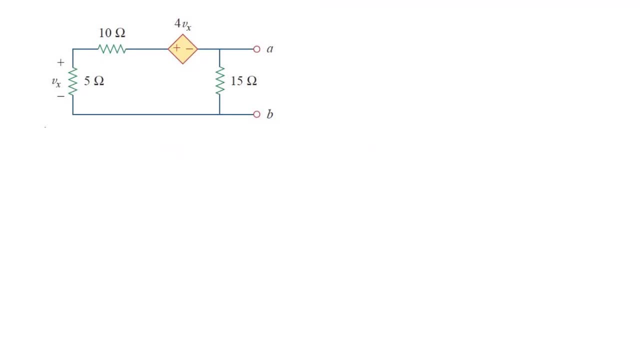 So negative 5 over 0 is equal to negative 1 over 5.. Negative 5 over 0 is equal to negative 1 over 10.. So Rth to be 1 over 5 is equal to negative 1 over 5.. 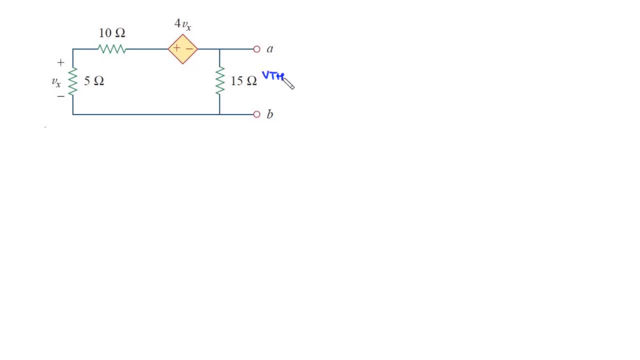 That's it. This is the porta-counsel voltage in the circuit And it's the voltage of the circuit. These are the voltage: Three volts. Let's move on to find Vth distribute current in this circuit. So we are going to consider current. 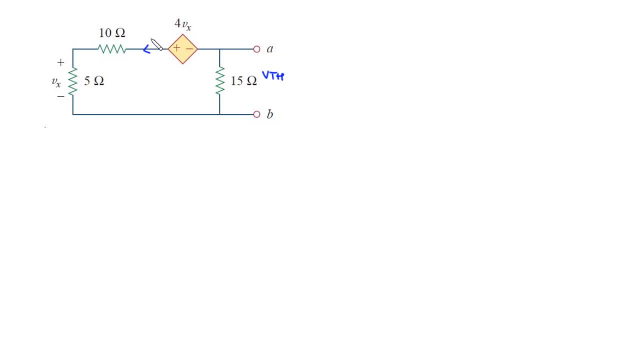 leaving in this direction And let's call that current Ix. So we have this Ix flowing through 10 ohms, 5 ohms and then 15 ohms. So we are taking the anti-clockwise direction. We have the source voltage to be. 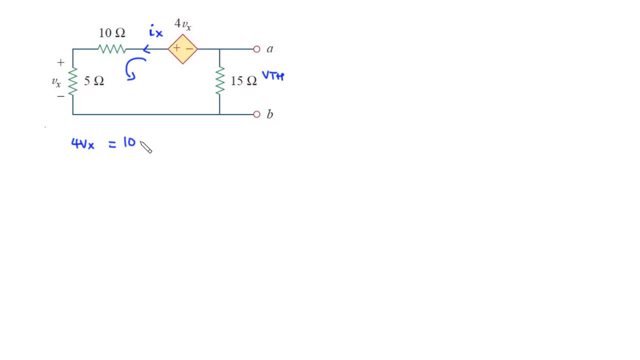 4Vx. That is equal to. we have 10 Ix plus 5 Ix plus 15 Ix. Now 10 plus 5 plus 15 is 30. So we have 4Vx equals 30 Ix Now. 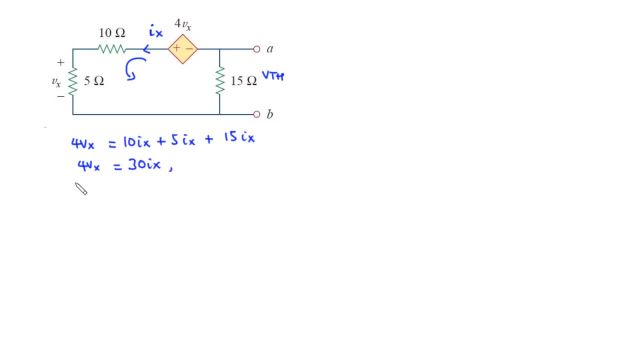 we have Vx to be the voltage across these 5 ohms, And then Vx is equal to the value of the current flowing through this branch, which is Ix times the value of the resistor. So that is: Vx equals 5 Ix, So that is the value of. 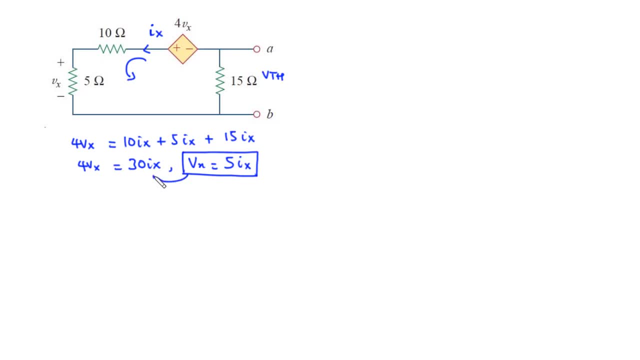 Vx, So let's substitute that into this equation. So we have 4 times 5 Ix equals 30 Ix. Now this becomes 20 Ix equals 30 Ix. We transpose this to the left hand side, we have 20 Ix. 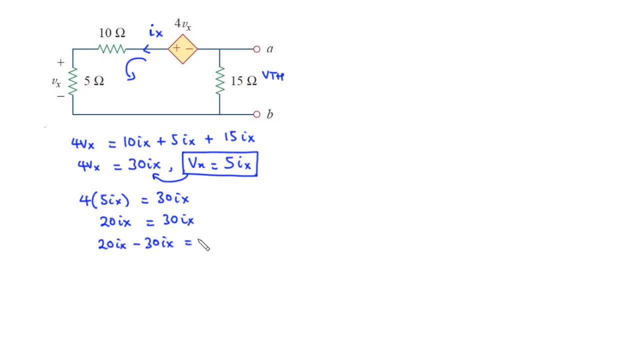 minus 30, Ix equals 0. So negative 10 Ix equals 0.. We divide through by negative 10, by negative 10, and then we have Ix to be equal to 0 A. So this is the value of Ix. 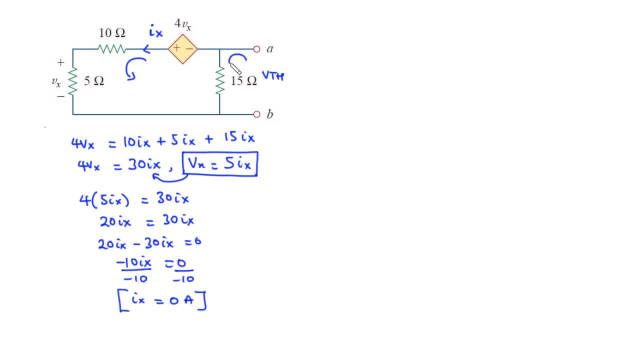 Now to find Vth, Vth, we are taking the anti-clockwise direction and Vth is equal to of the current flowing in this branch, times the value of the resistor. now we have the current flowing through this branch as IX, and then we are taking the.